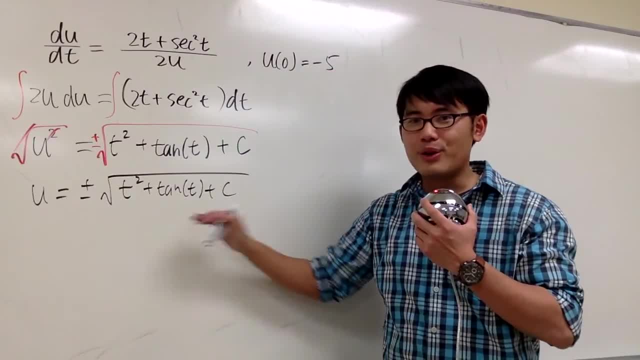 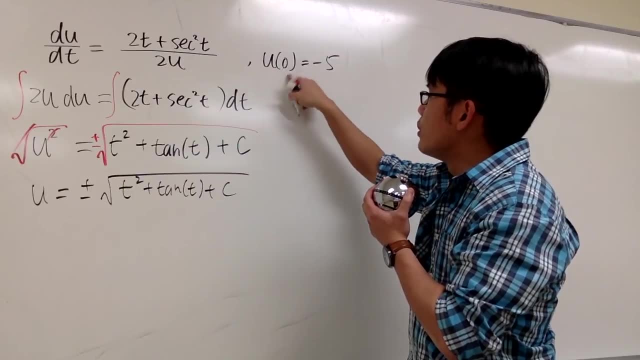 We must make sure that this initial condition comes to play right here with our equation that we have With. that being said, this initial condition means we have u of 0. That means, when t is equal to 0, we must have the u for u to be negative 5.. 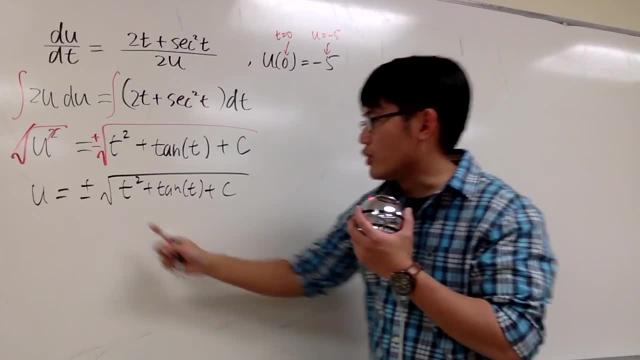 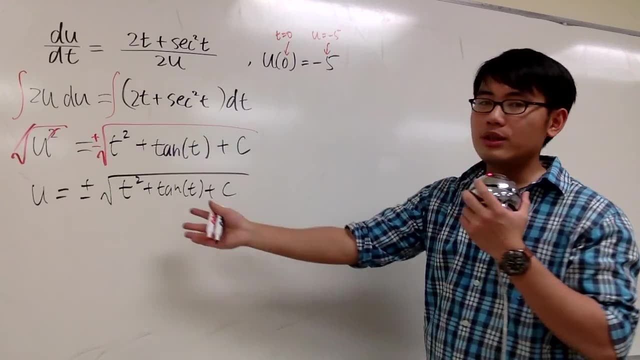 And with this initial condition we can also make a decision on should we keep the plus square root or should we keep the minus of the square root. So let's just plug in the values into u and t. Negative 5 goes into the u. 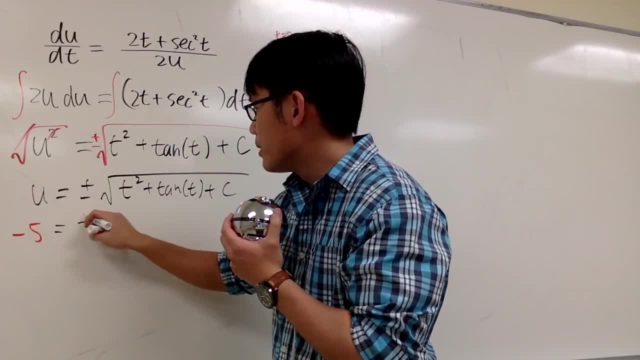 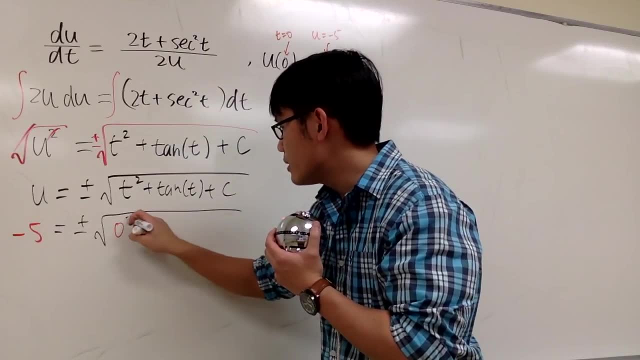 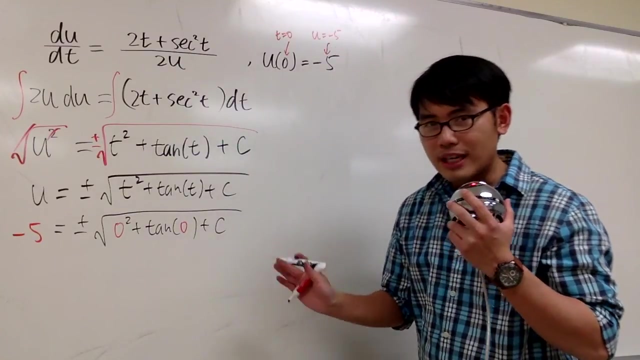 So let me write down negative 5, and this is equal to plus or minus. square root of plugging t is equal to 0,. okay, So we have 0 squared plus tangent of 0 plus c, And now can we make a decision on: should we keep the positive? 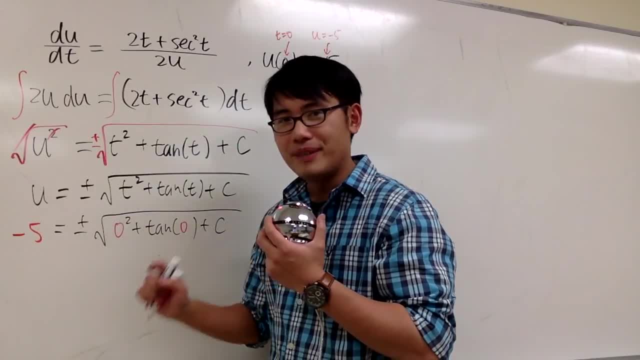 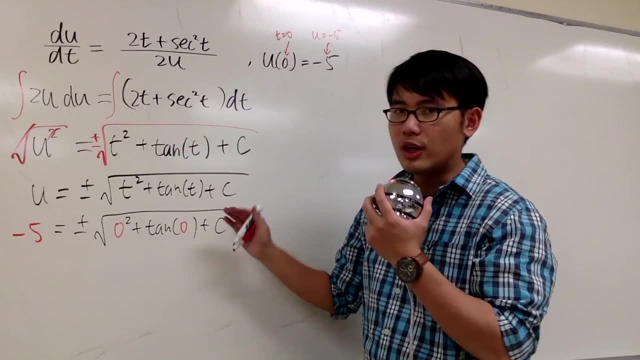 or should we keep the negative? We should keep the negative because on the left-hand side we have a negative already. This is a negative 5. And remember, the output of a square root is always going to be positive, So we are going to actually get rid of the positive version. 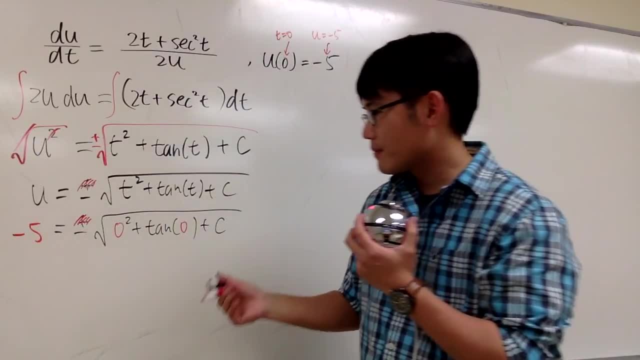 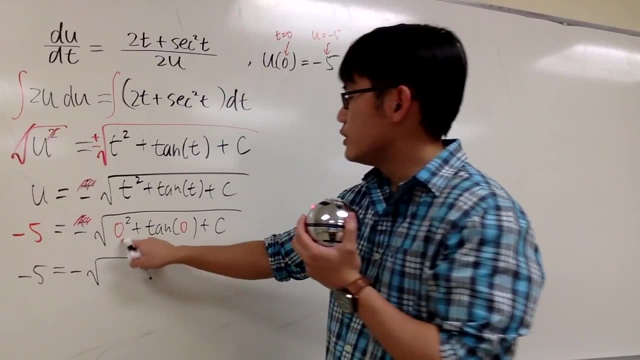 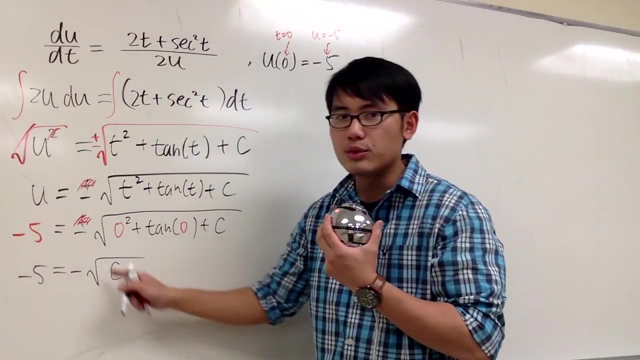 This way, negative matches negative okay, And we will see that we have negative 5.. This is equal to negative square root. 0 squared is 0, tangent 0 is 0, and we just have a c. Negative 5 is equal to negative square root of c. 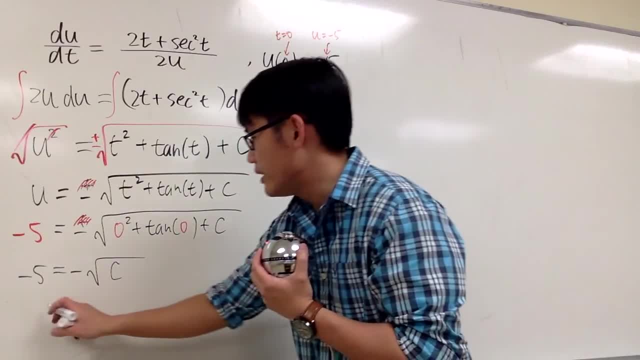 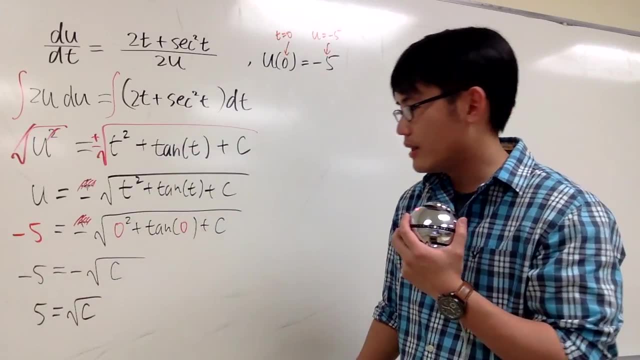 Of course we can divide both by a negative 1, and we end up with positive. 5 is equal to positive square root of c. after we get rid of the negative on both sides- And we can square root both sides- we get c is equal to positive 25.. 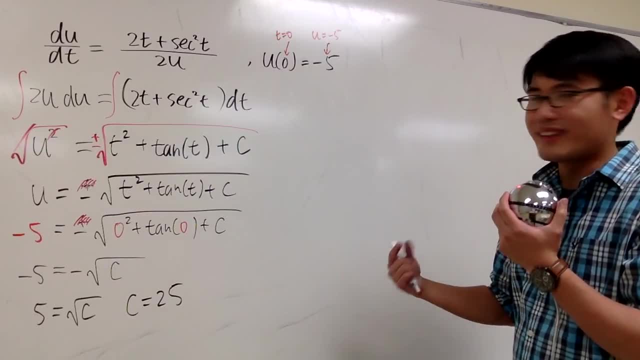 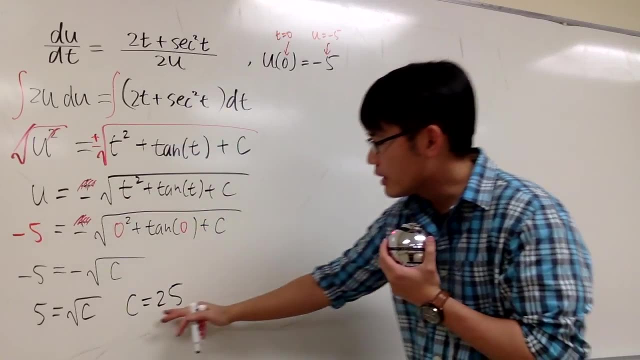 Well, we get a c, and now this is how we are going to write down the answer. This is the general form, where we got rid of the positive version already, And I just have to plug in 25 into the c right here and that will be the answer. 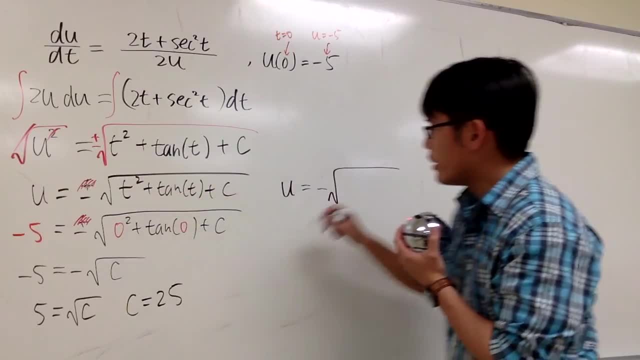 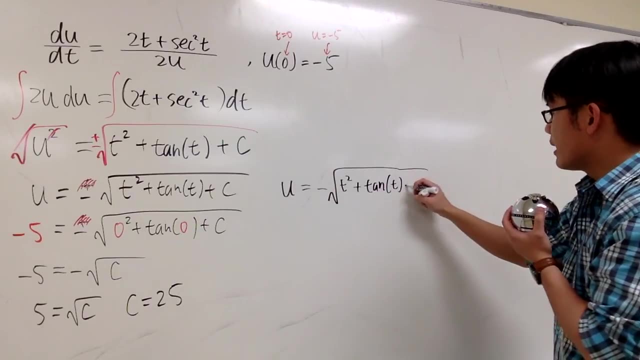 u will be negative. square root t squared plus tangent of t and the c value is equal to positive 25.. And this, right here, is the answer. That's it.